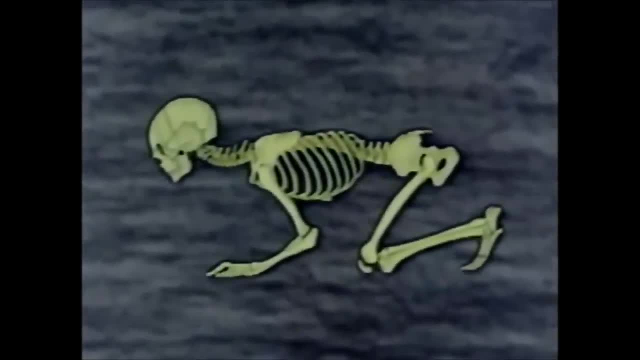 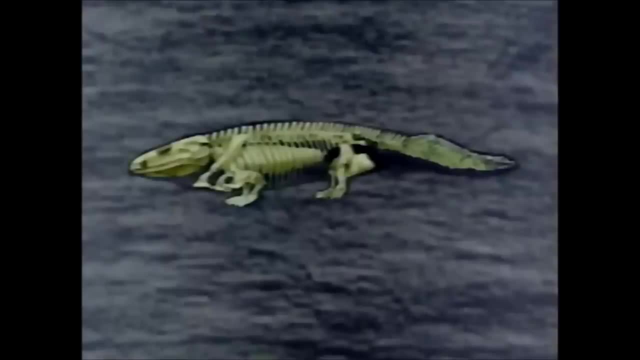 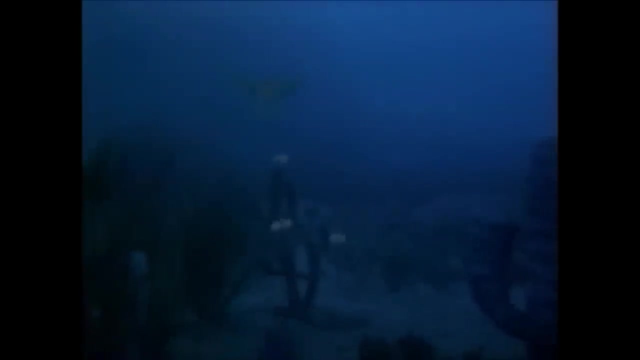 Though much about our lineage remains a mystery, the origins of the human backbone are linked to pikaia and its notochord Few. developments would lead to greater diversity. The reign of Anamalocaris was not short-lived. It flourished. 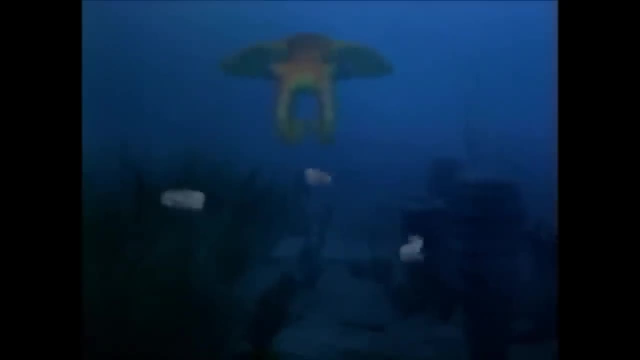 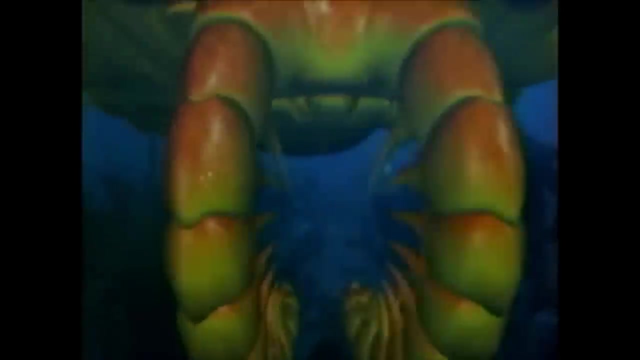 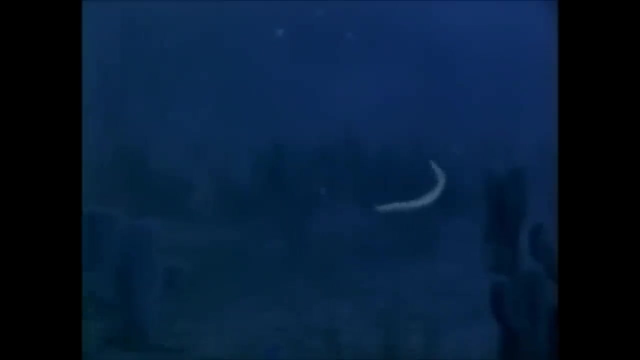 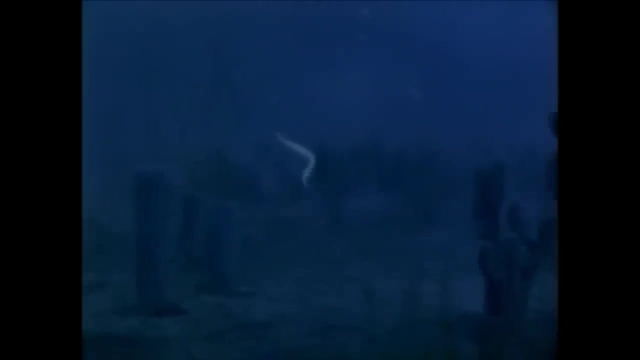 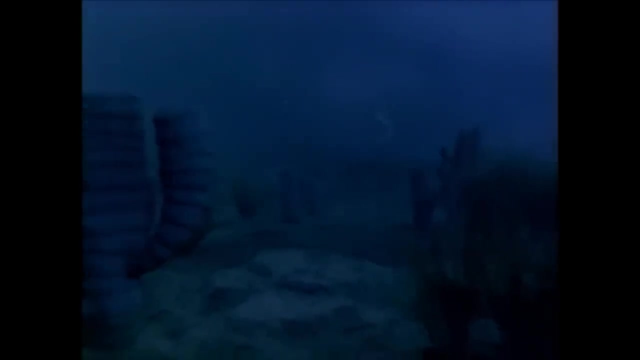 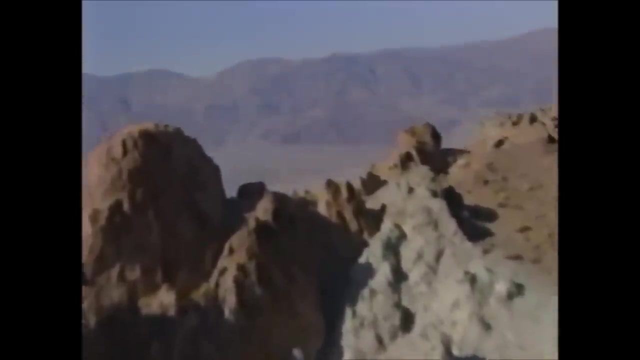 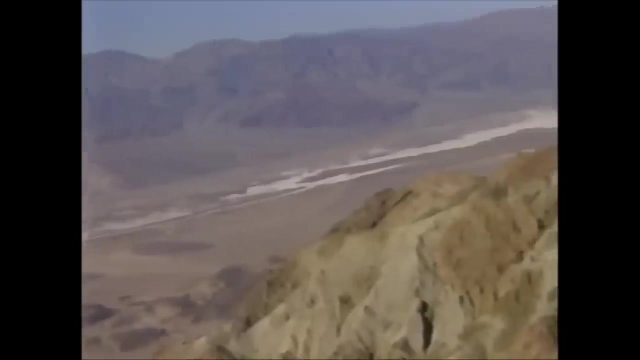 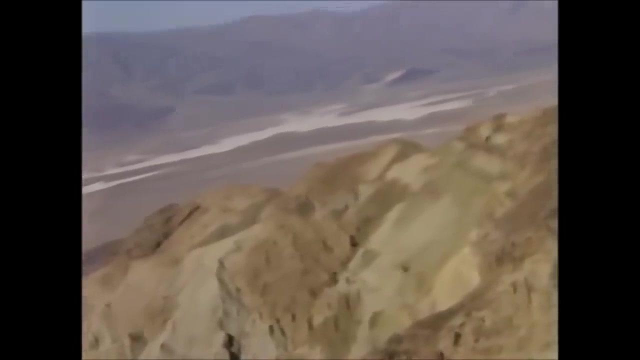 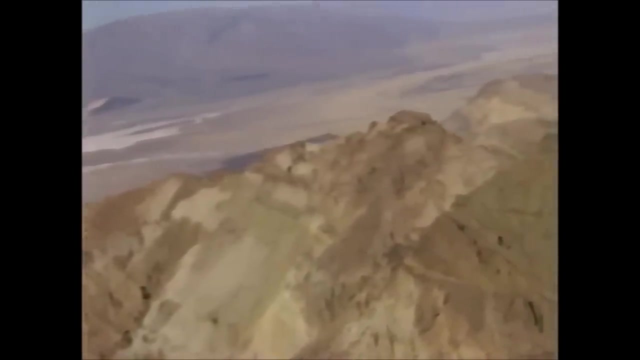 that would eventually populate the seas, the land and the skies. California's Death Valley- one of the most arid regions in the world. California's Death Valley- one of the most arid regions in the world. It was here that the fossils of the first fish to brave the freshwater habitat were found. 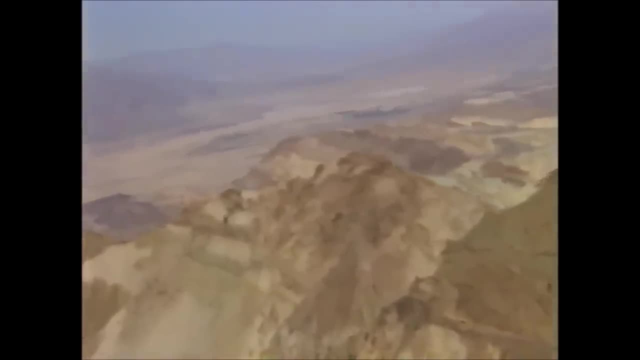 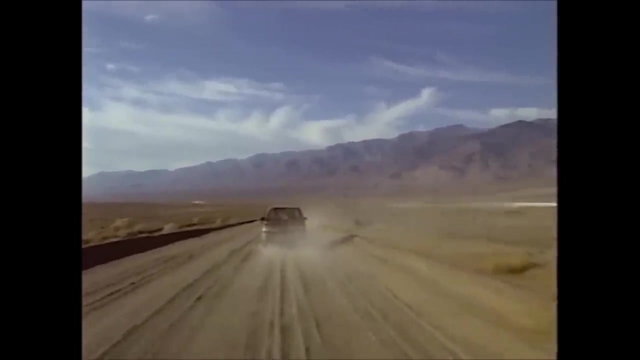 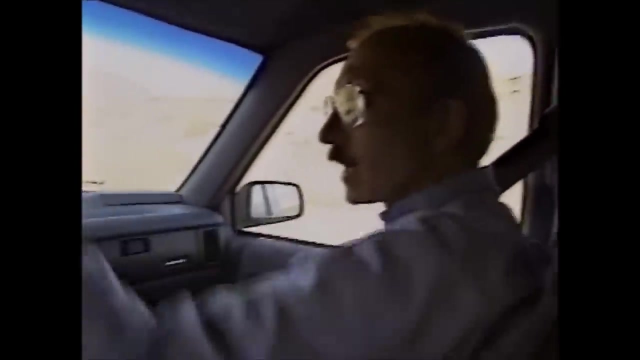 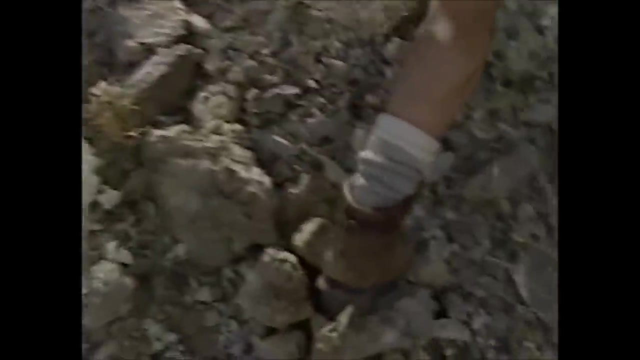 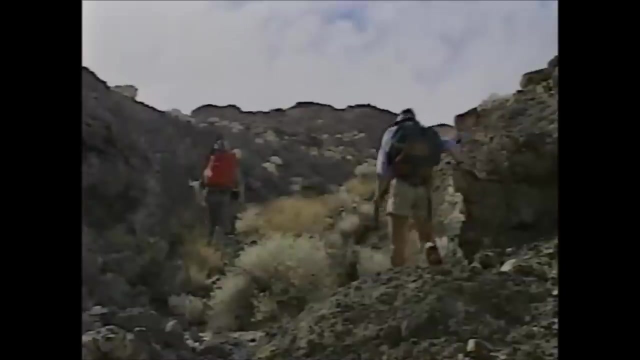 It had taken them 60 million years to gain access to these estuaries. The man who discovered the fossil was Dr David Elliott of Northern Arizona University, a specialist on ancient fish. Tons of earth and sand formed sediments at this site, deposited by the river that ran through Death Valley eons ago. 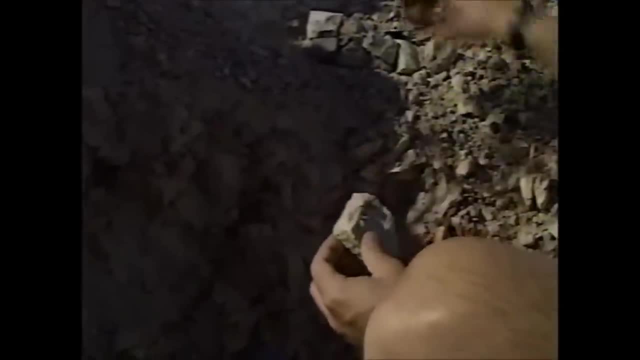 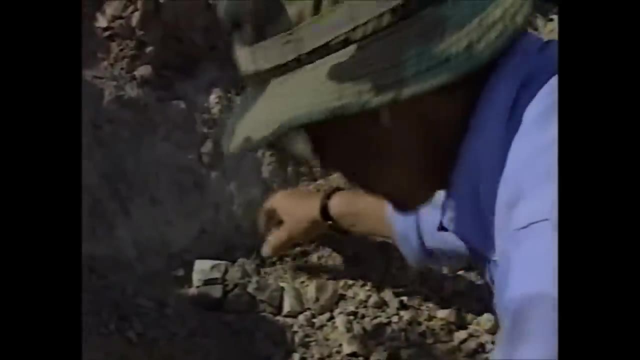 And it is here that Dr Elliott has been focusing his excavation and research work on ancient freshwater pioneers. I can't really tell what that is. This is a teraspid, this is a lingulid And this is a teraspid. 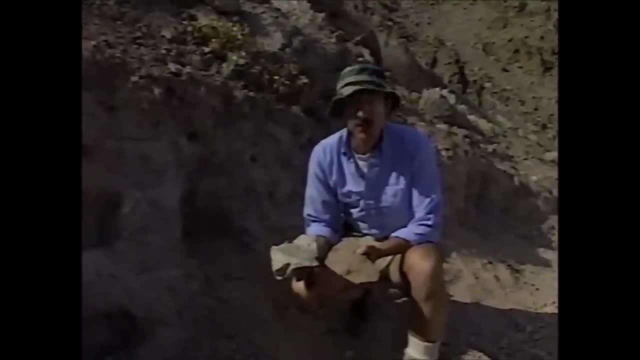 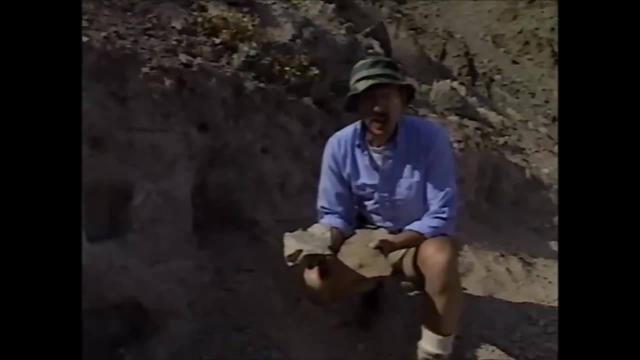 And this is a teraspid- And lingulids are rather interesting because they're characteristic of estuarine environments, that is, environments in which freshwater and marine waters are mingling. These are areas of very high nutrients where you may have large numbers of organisms coming to feed. 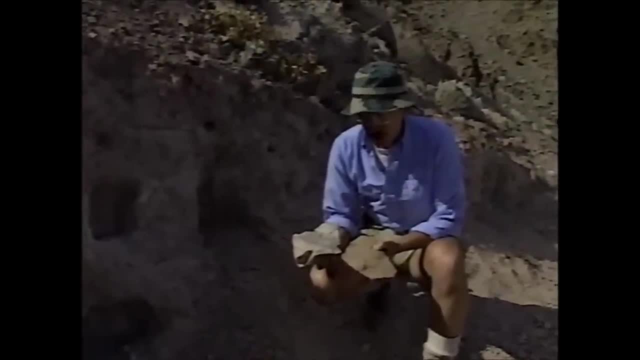 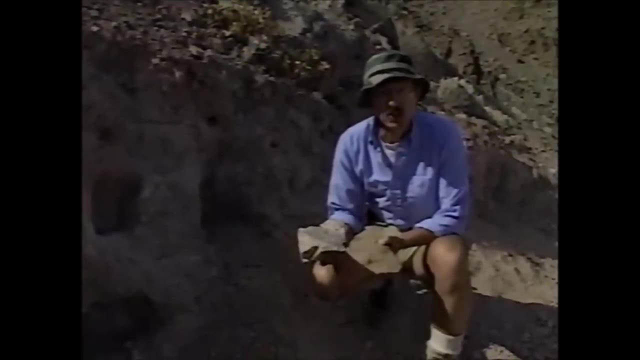 and we have many teraspids here. There are also areas that many marine organisms can't get into. They're not able to survive in brackish conditions, and so it may be that teraspids were protected- protected from some of their possible predators- by living in these environments. 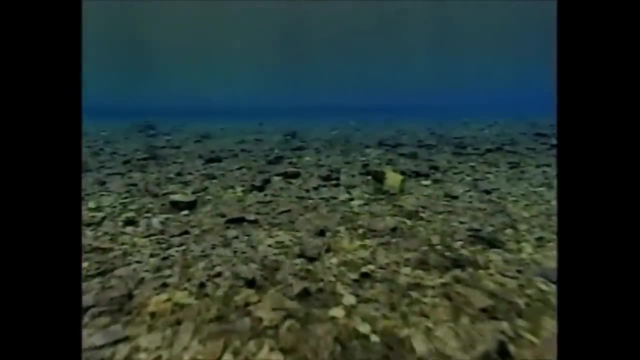 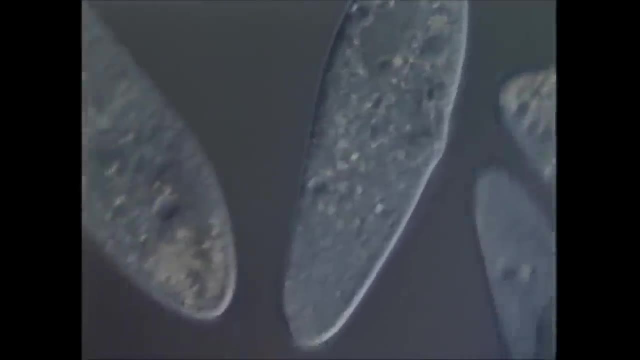 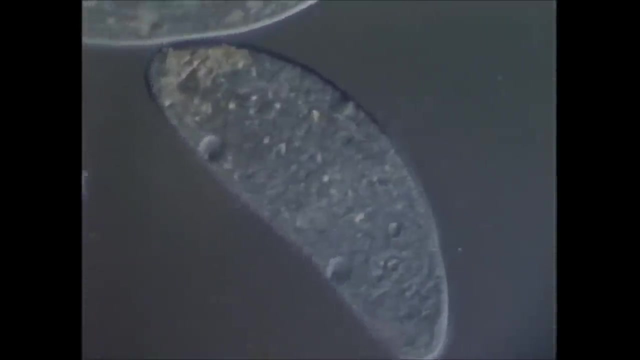 Freshwater habitats have almost no salt content. A change in salinity can spell instant death for unacclimated marine life. This paramecium thrives in the salty medium of seawater Breathing saline fluid. it regulates its mineral levels and ejects wastes. 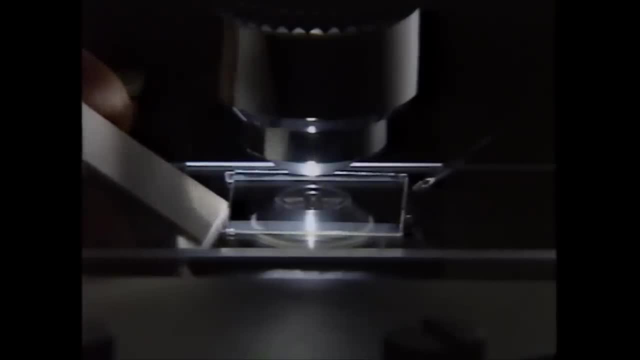 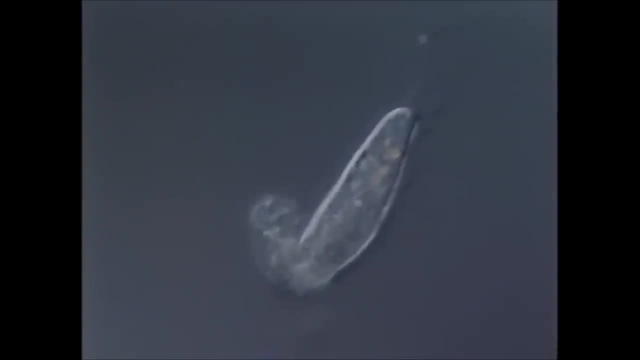 Salt free marine life is not limited to salt Free water is added, changing the balance In this unfamiliar, hostile freshwater environment. the paramecium takes in water without voiding it, destroying the cell. The now bloated paramecium ruptures and dies. 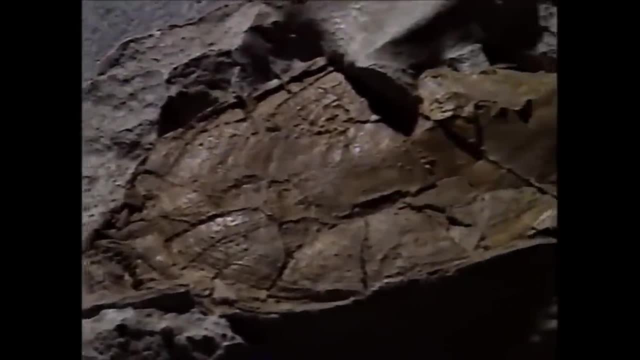 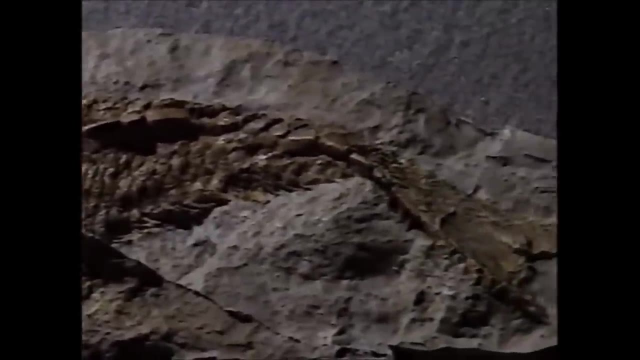 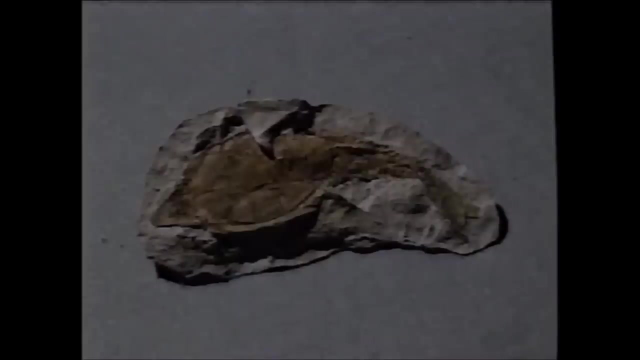 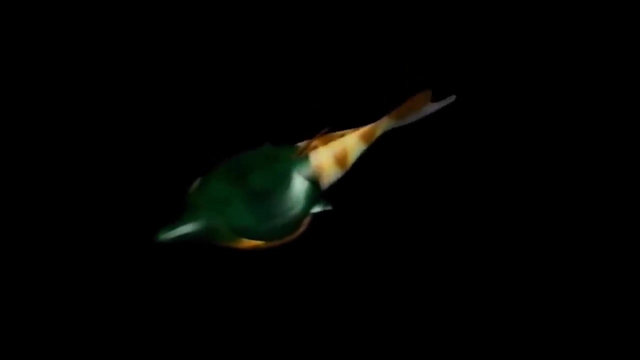 Teraspis is about eight inches long, its head covered with tough bony armor and its body with primitive scales. Unlike paramecium, teraspis managed to adjust to this new freshwater habitat with a little creative bioengineering. Music plays. 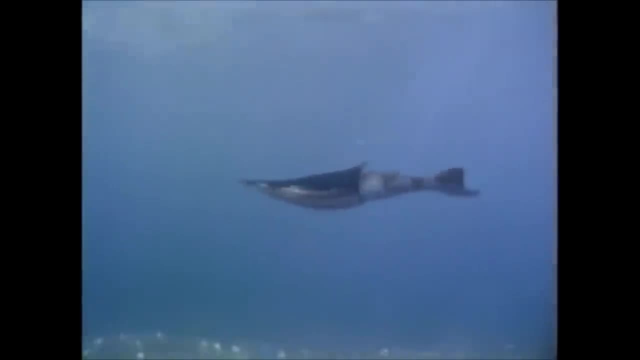 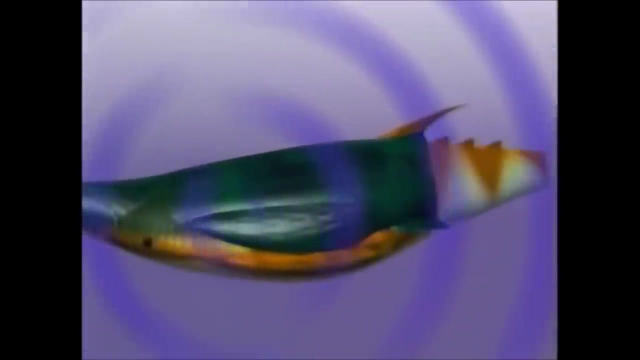 The teraspid's protective shell prevented water from penetrating the body through its outer layers, But the gills it used to breathe were a weak spot. Music plays To balance its system. teraspis developed a kidney powerful enough to pump extraneous water from its bloodstream. 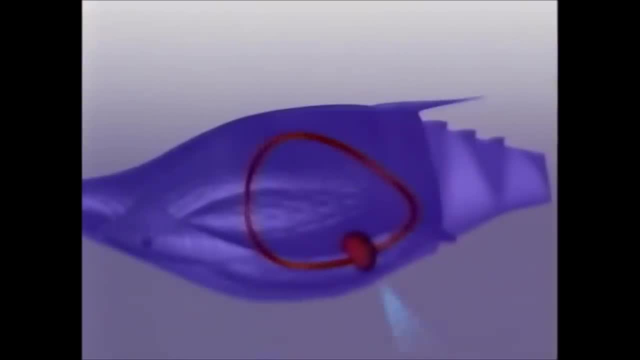 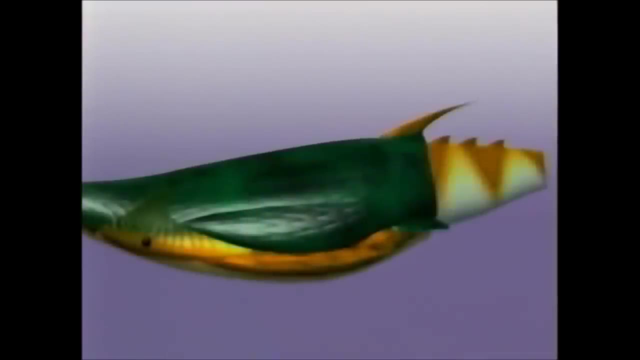 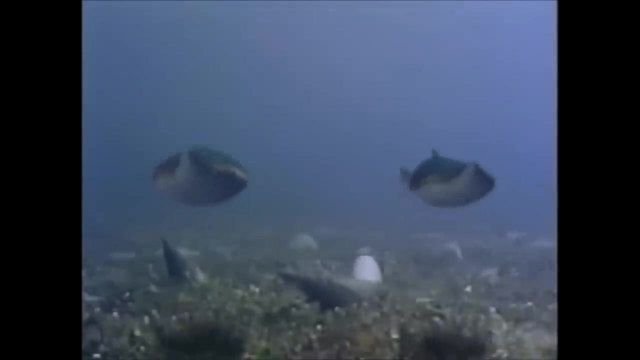 Music plays. Transforming its physiology was a major evolutionary breakthrough for the first freshwater fish, But it was only a first step. Music plays. 400 million years ago, life on the river was unfolding- Music plays. But the freshwater habitat posed new challenges. Music plays. 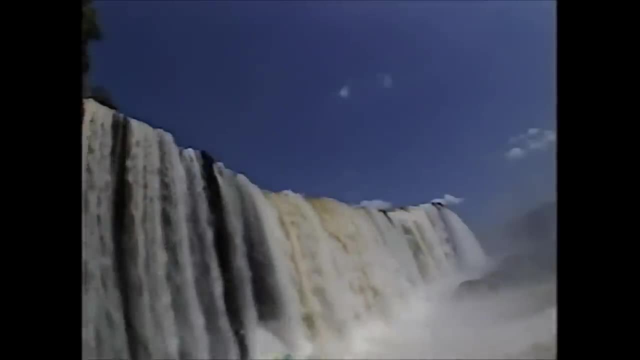 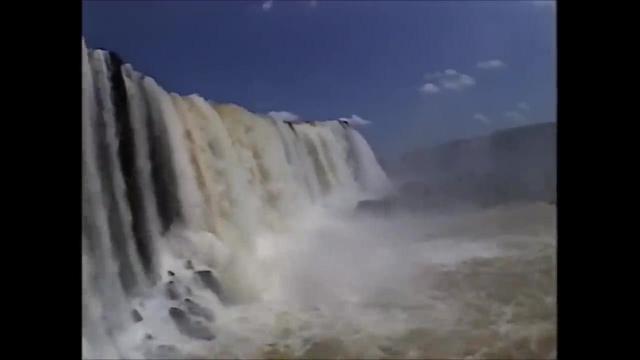 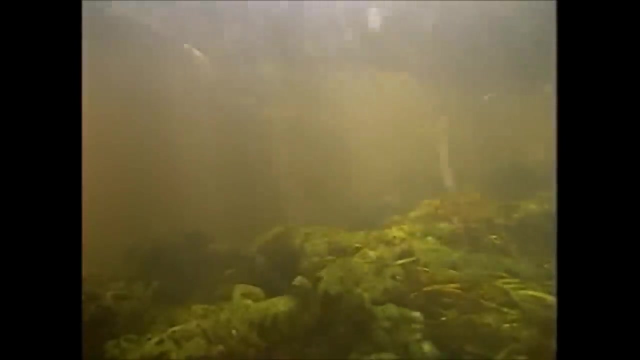 Rapid currents and waterfalls to negotiate Music plays. It took millions of years for marine life to adapt to these new ecosystems. To survive here, Earth's first fish would experiment with many anatomical designs- Music plays. The Miguasha Park lies on northeastern Canada's Gaspé Peninsula. 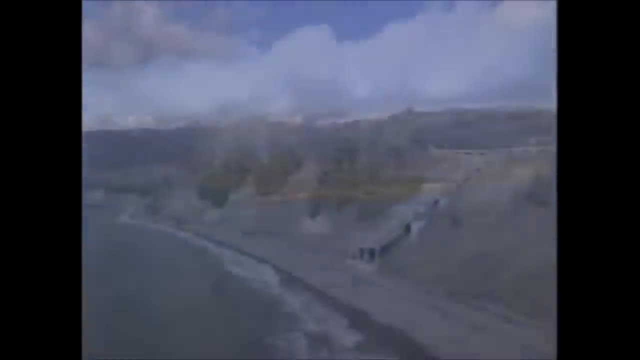 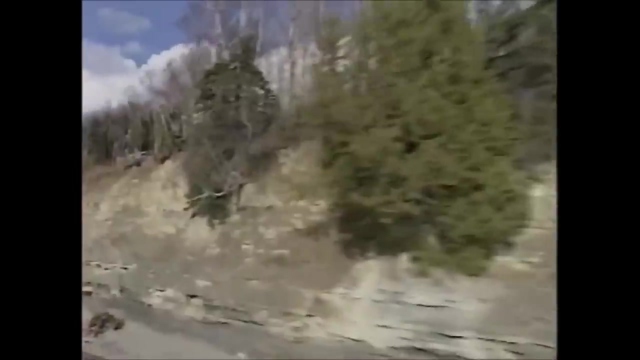 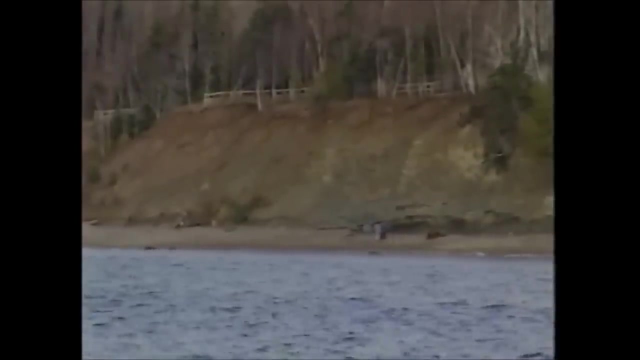 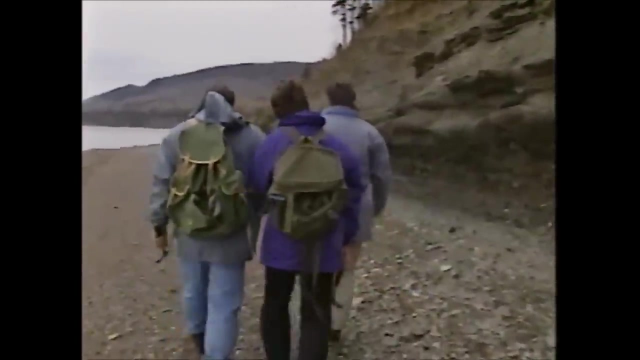 Music plays. 400 million years ago, this was a tropical region situated directly under the equator. Music plays: Hedged in this meandering stretch of cliffs is the 20 million year history of fish evolution. Music plays Fossils of freshwater pioneers. 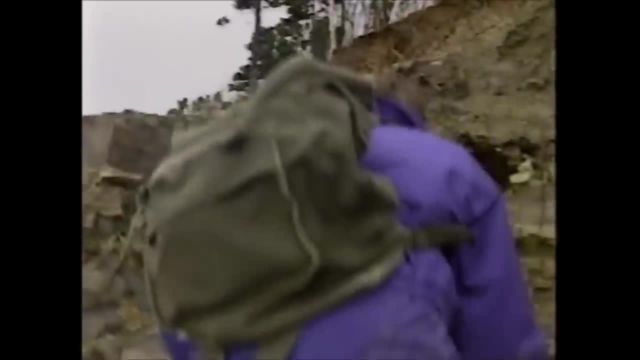 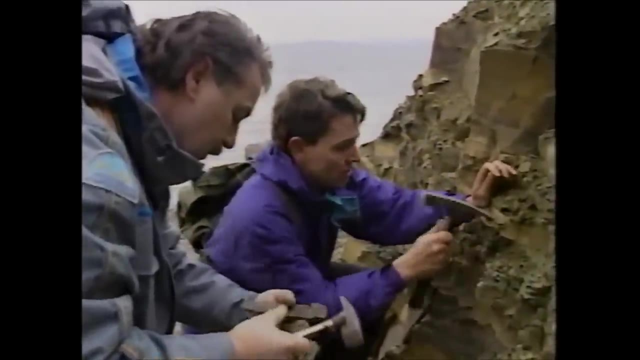 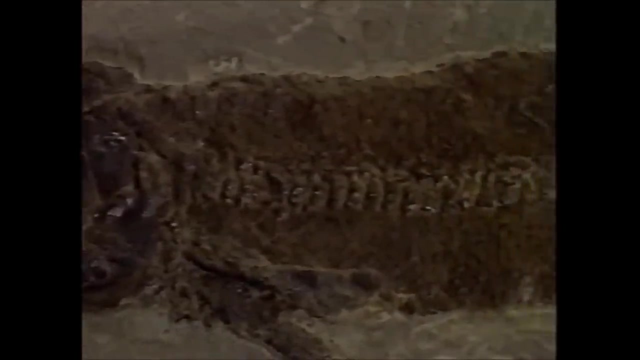 Music plays Fish with fins to resist river current. Music plays Carnivorous fish with jaws and teeth. Music plays. There's some layers with more aspenusias Music plays. And a peculiar fish entirely different from any of the others Music plays This fish had a backbone. 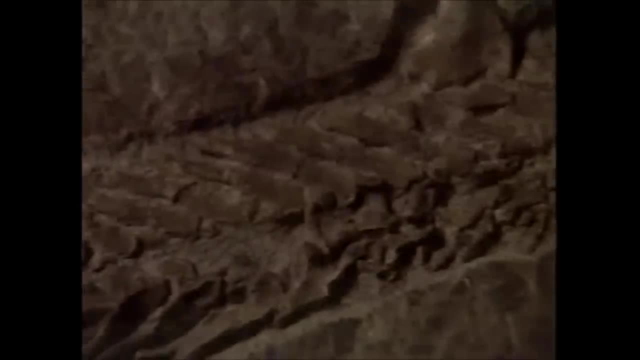 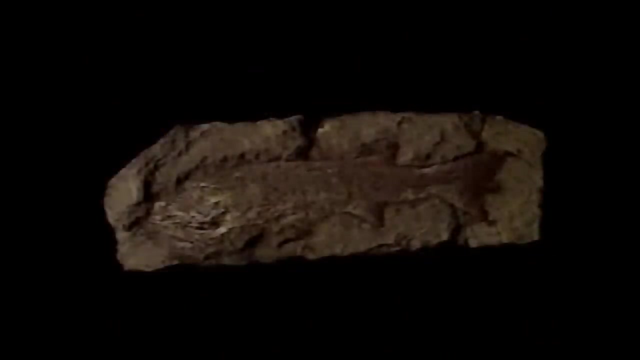 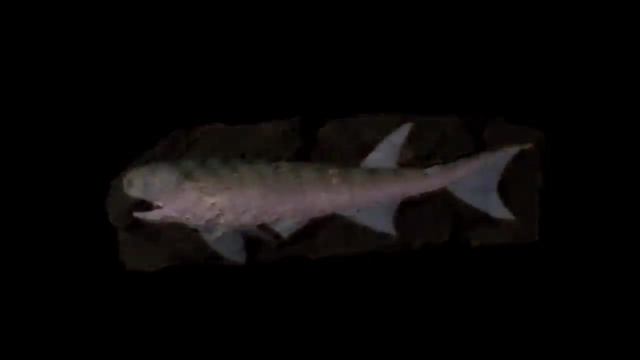 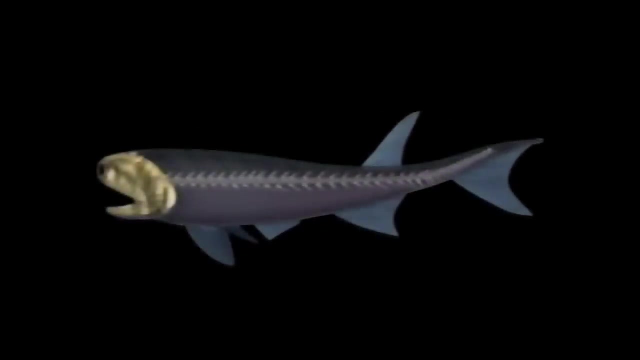 Music plays, Music plays. Until now, there were fish with tough exoskeletons- Music plays- But none with hard bone inside the body. Music plays Carolepis, the earliest creature with a spine, appeared 390 million years ago. Music plays The most common fish today. the bony fishes are its direct descendants. 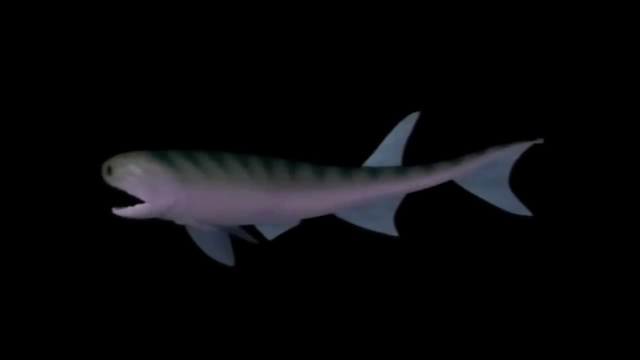 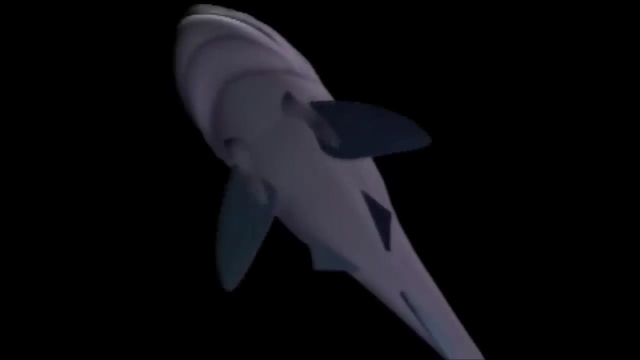 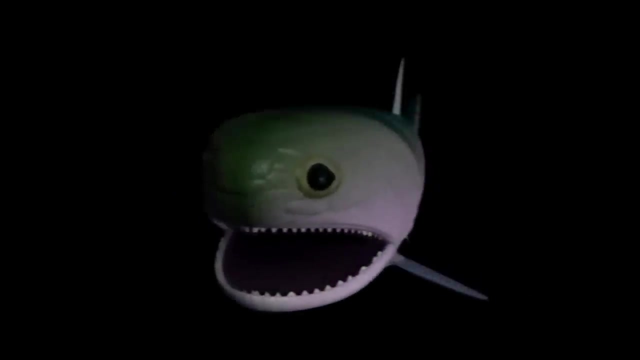 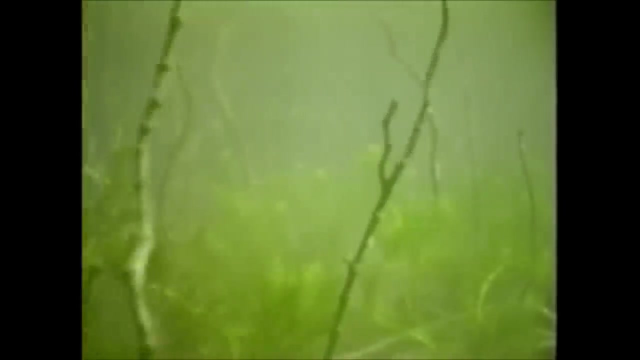 Music plays. Like modern fish, Carolepis was equipped with one pair each of pelvic and pectoral fins. Music plays: It was sleek, with jaws and sharp teeth for catching prey. Music plays: Acquiring a spine, Carolepis developed strong muscles to swim with speed and power. 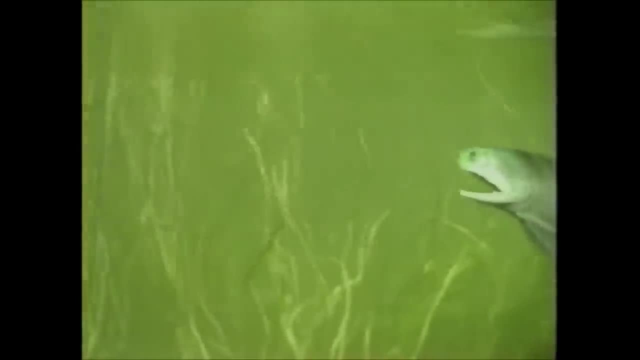 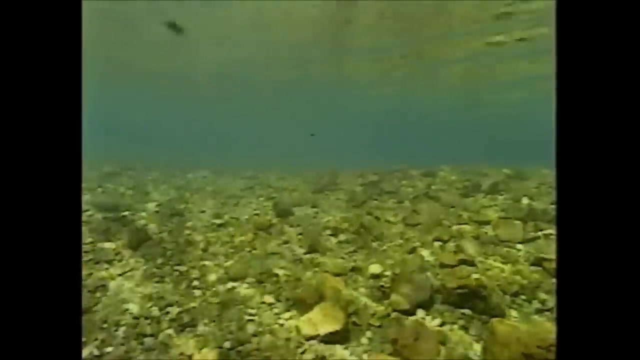 Music plays. But there were other agile swimmers in the river that had managed to do without one Music plays. Why, then, did the backbone develop Music plays? While the sea was rich in minerals essential to life, the river was in short supply. 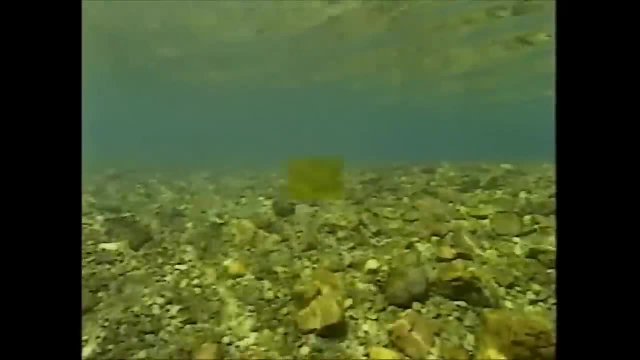 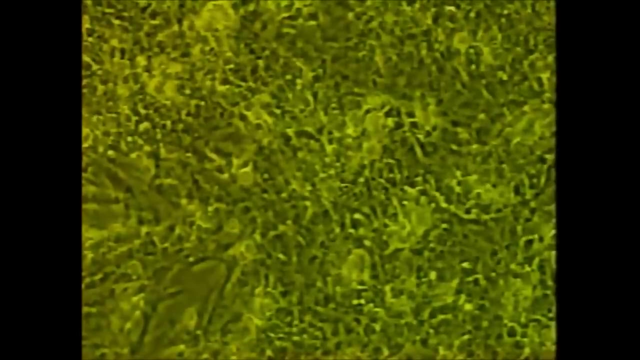 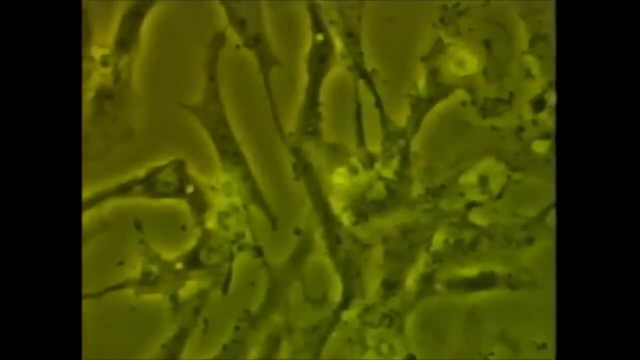 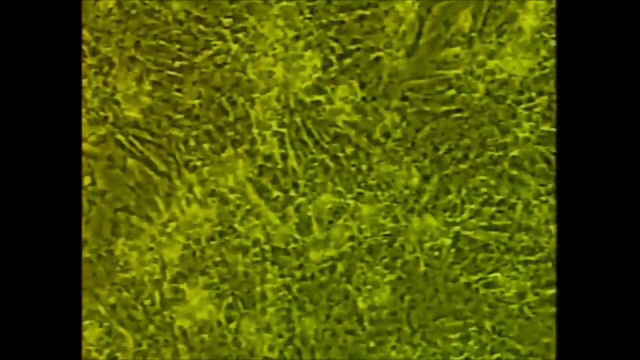 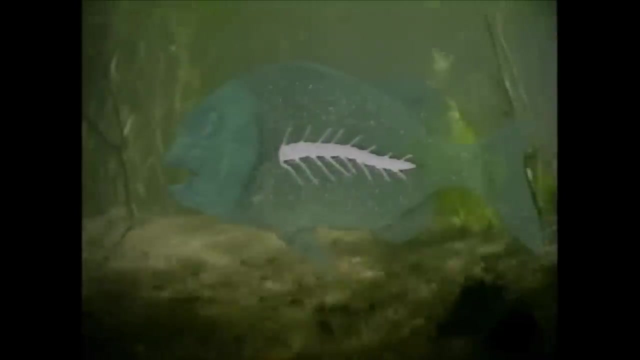 Music plays. This is heart tissue. Music plays. Working in unison, these cells allow the heart to pump blood throughout the body. Music plays. To function properly, the heart needs calcium. Music plays. Calcium concentration in a river is in perpetual flux. Music plays. 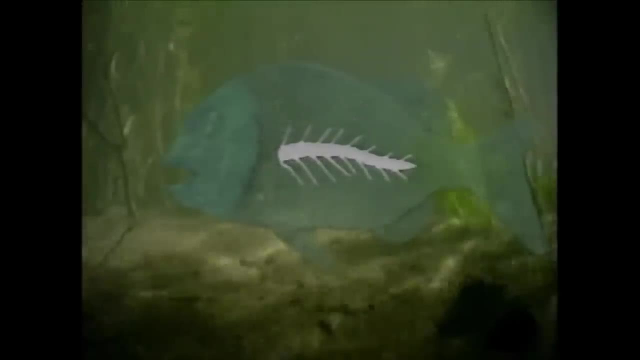 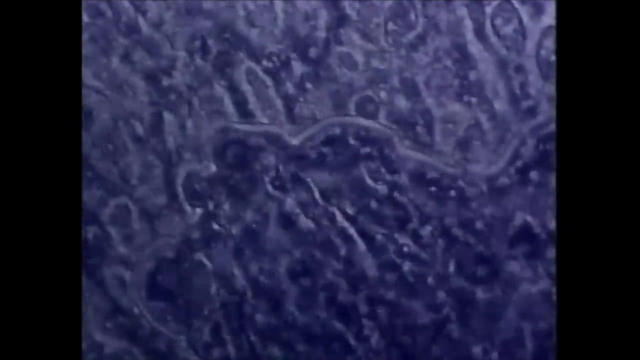 When levels are high, calcium is stored as bone Music plays. When they're low, the bone reservoir supplies the necessary mineral regardless of external conditions. Music plays. Meanwhile, the seemingly solid bone is constantly being replenished. Music plays At the top of the screen, hard bone is visible. 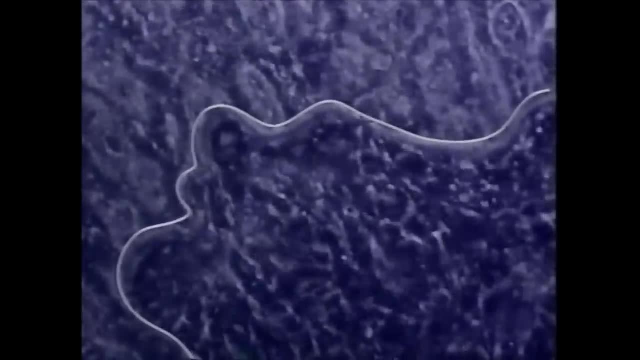 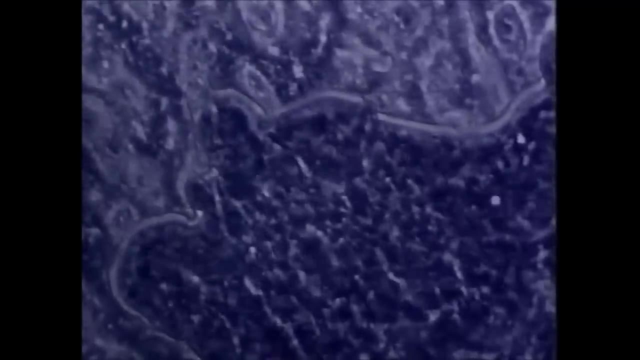 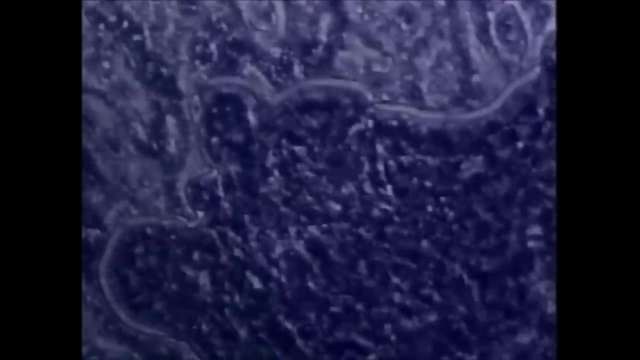 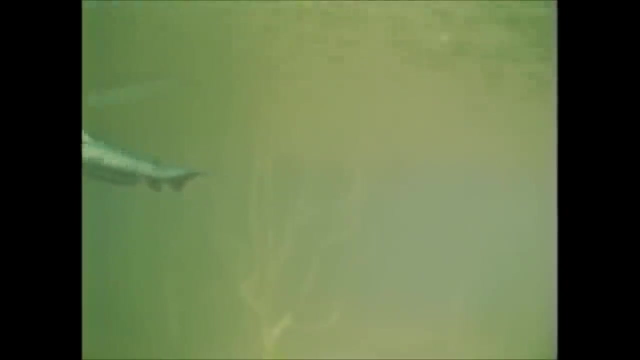 Music plays Moving below are cells that dissolve it. Music plays: Once the bone is dissolved, calcium circulates through the bloodstream to every part of the body. Music plays The fate of ancient fish rests on a simple backbone. Music plays Those without eventually perished from calcium deficiency or returned to their native sea. 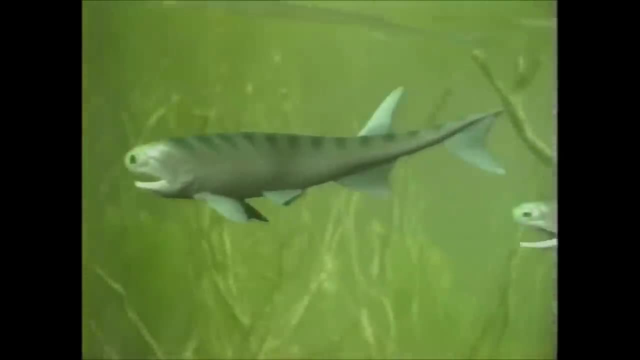 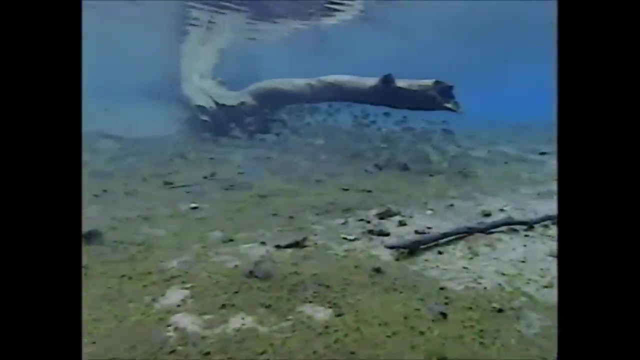 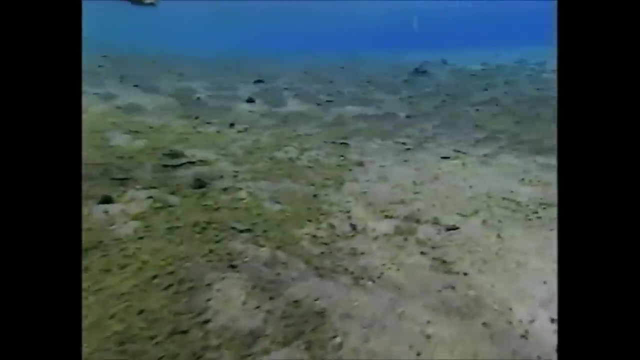 Music plays. For many years, Cairo Lepus reigned as the king of freshwater fish. Music plays. His anatomy gained him independence from the marine world. Music plays, Music plays. The descendants of Cairo Lepus thrive in both fresh and saltwater habitats. 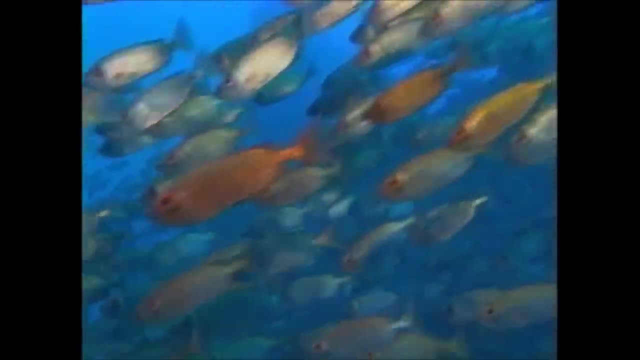 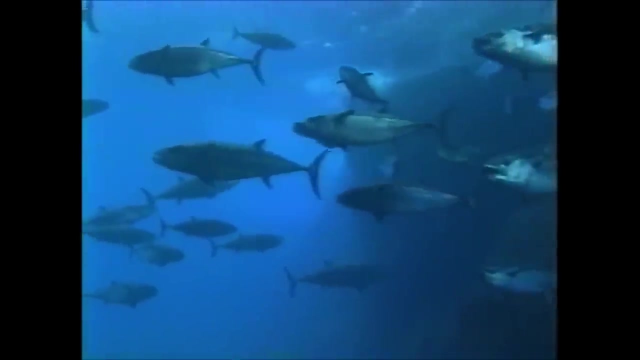 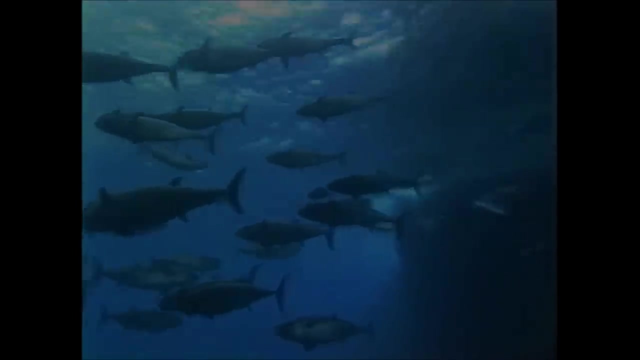 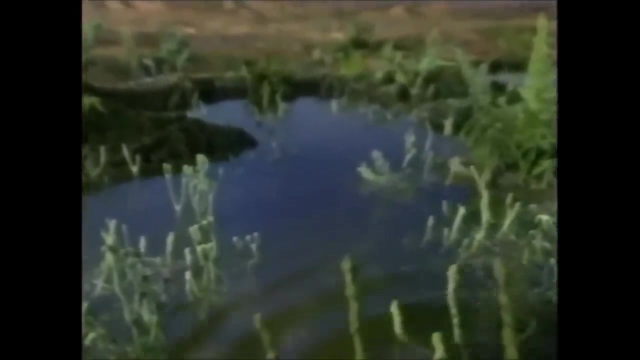 Music plays. The river was a proving ground for the earliest fish and their offspring, Music plays, And in this new habitat they gradually adapted the body system's key to survival on land. Music plays- Music plays. Another fish with a backbone appeared on the river at about the time of Cairo Lepus. 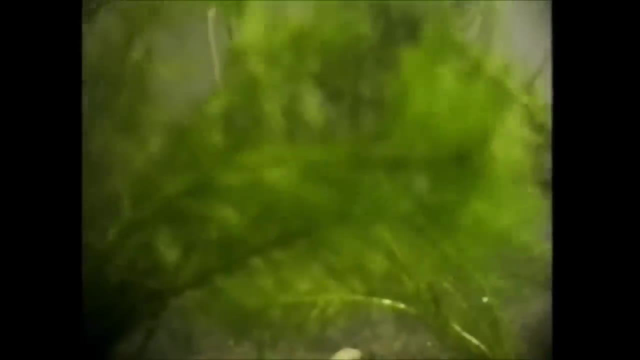 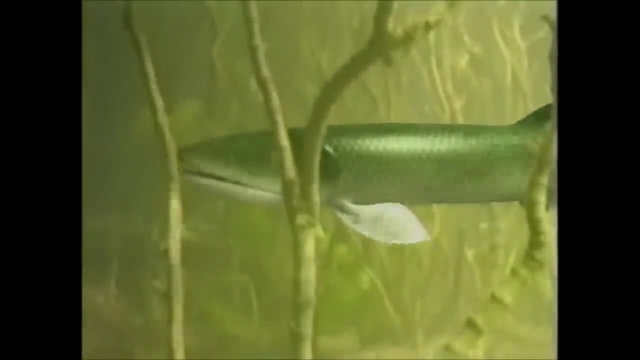 Music plays. It was called Eusthenopteron, a bottom dweller, Music plays. Eusthenopteron was not an efficient swimmer like many fish, but it had secured an evolutionary niche with powerful bony fins to push its way through the river's undergrowth. 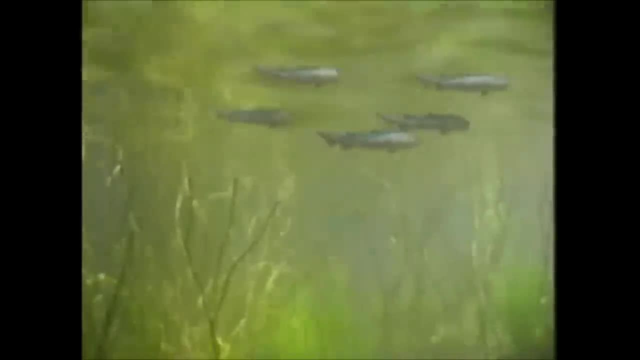 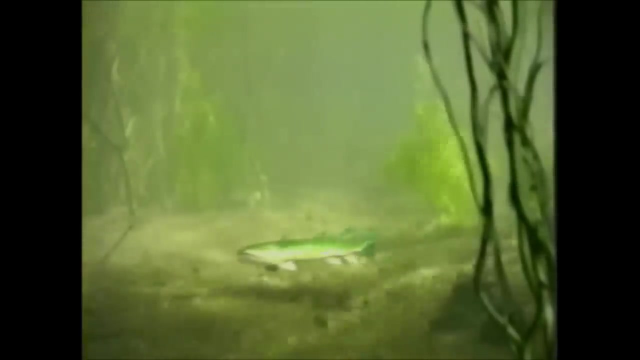 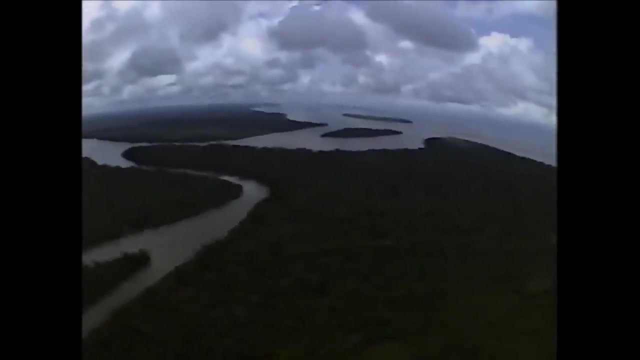 Music plays. This fish was a stealthy hunter poised for action. Music plays Eusthenopteron's habitat shaped its unusual bone structure, which would one day lead to the evolution of terrestrial animals. Music plays: South America's Amazon breeds acres of jungle swampland. 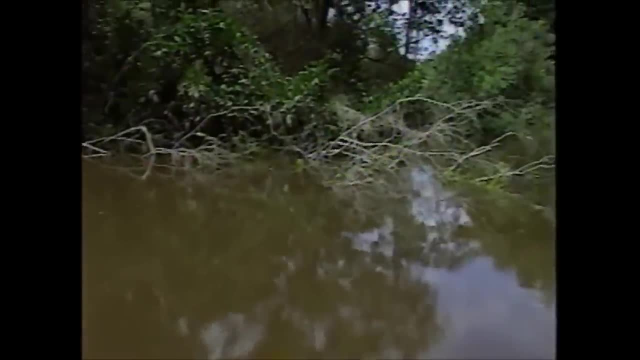 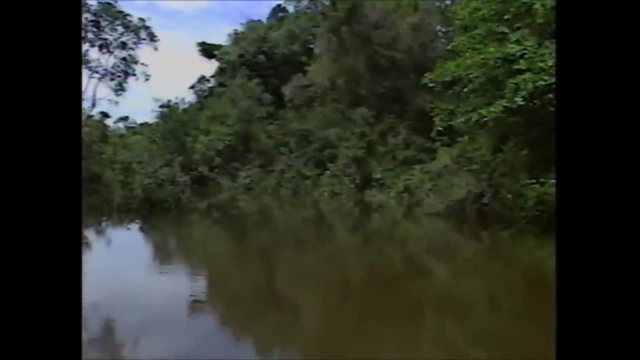 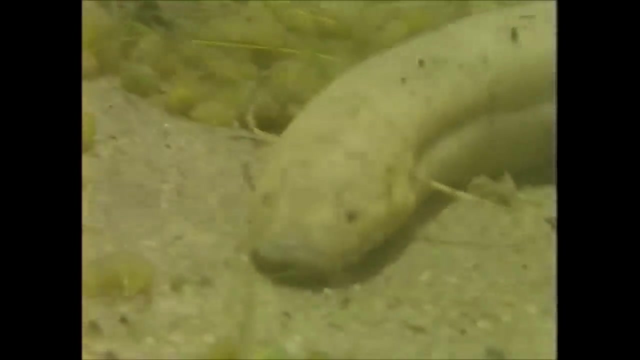 mimicking conditions in the age of Eusthenopteron, Music plays. And with the swamps, a host of unusual life forms Music plays. Among them, the lungfish, a mud-dwelling creature, Music plays. This fish has gills, but it also has lungs for breathing air. 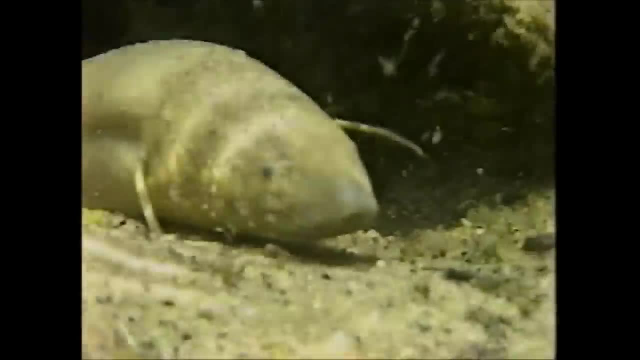 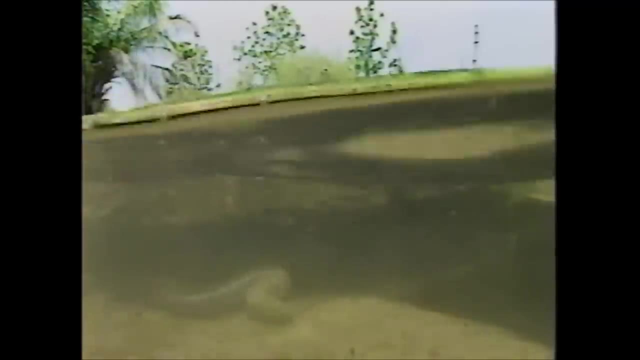 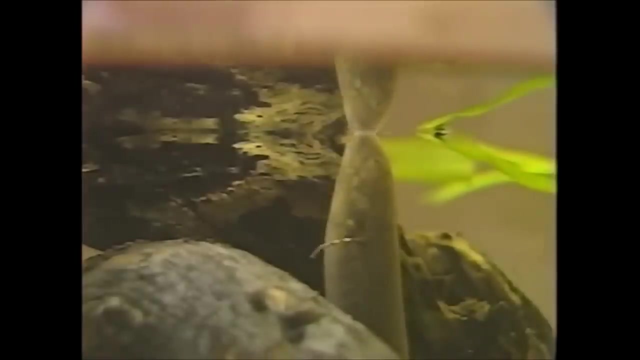 Music plays. In such murky water, oxygen content is often very low. Music plays: The lungfish probably developed lungs to breathe oxygen from the air when the supply in the water was depleted. Music plays Just as its ancestor, Eusthenopteron had done eons before. 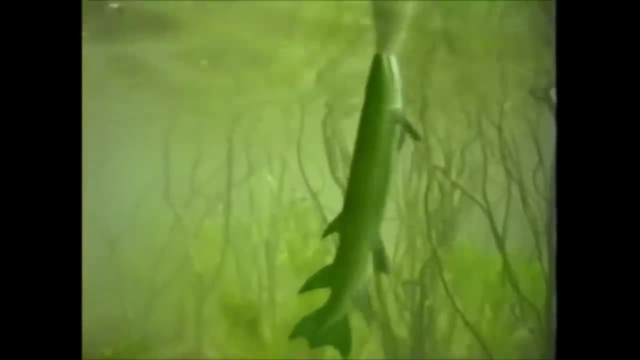 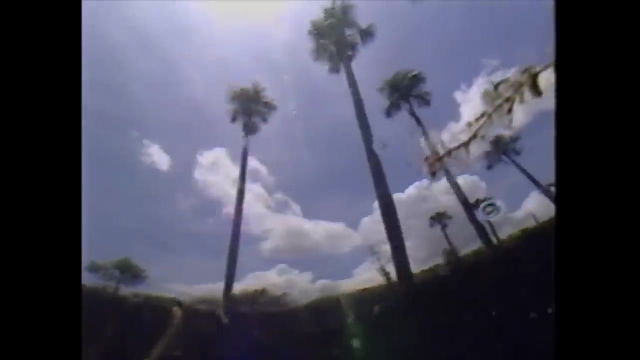 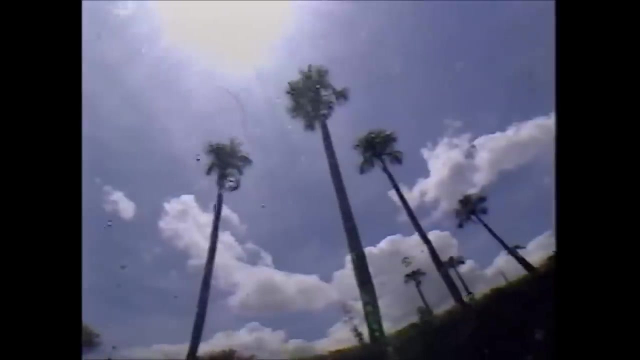 Music plays. Poking its head above the surface for a life-sustaining breath, Eusthenopteron surely caught a glimpse of the world above the waterline. Music plays Now that fish had evolved kidneys, bone and lungs. land was almost within reach. 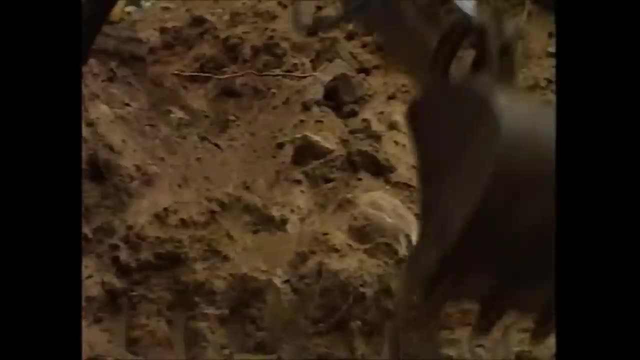 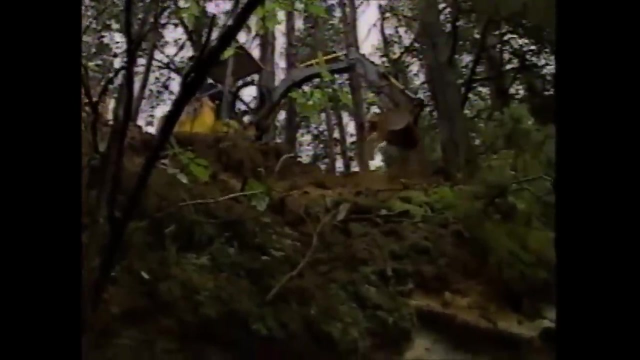 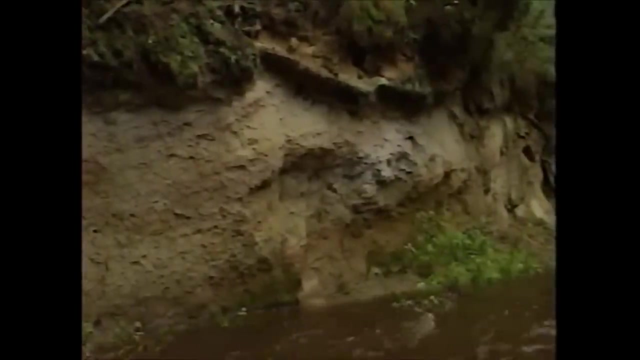 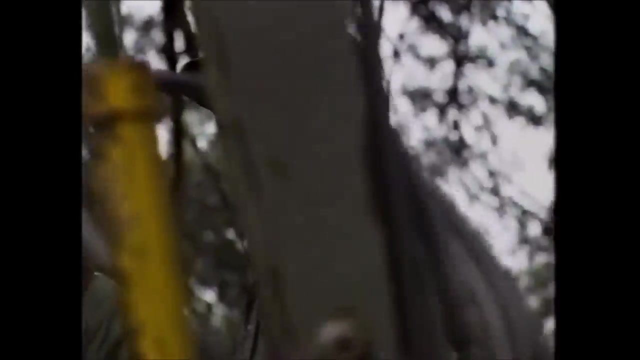 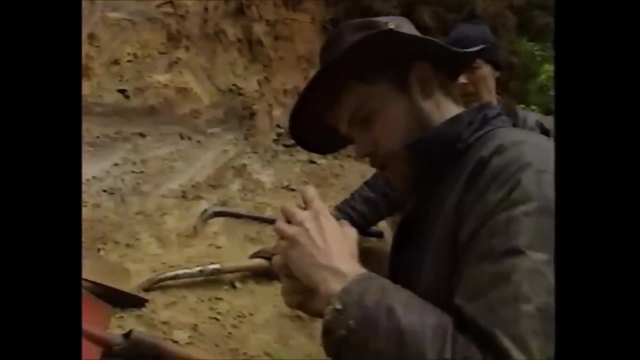 Music plays. The first four-legged creature appeared 10 million years after Eusthenopteron. its remains discovered in a forest in Scotland. Music plays. At the time this region resembled today's Amazonian swampland. Music plays Dr Per Erich Ahlberg of the British Natural History Museum. 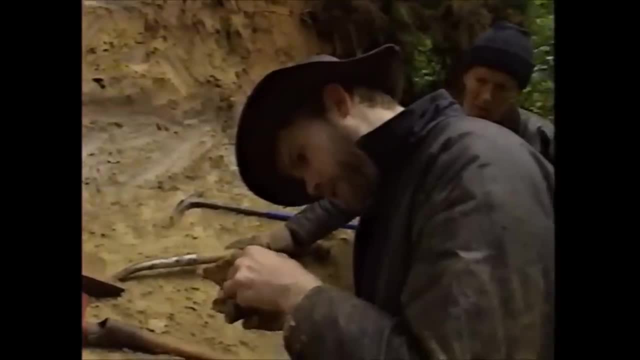 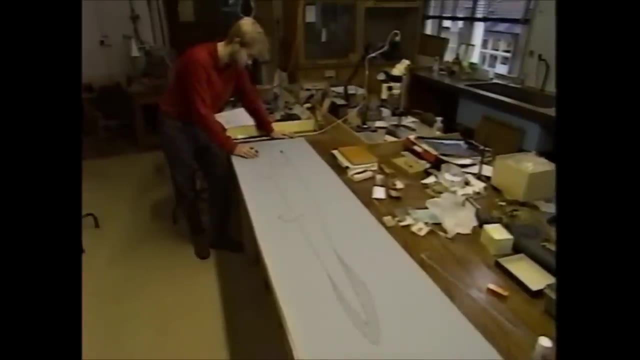 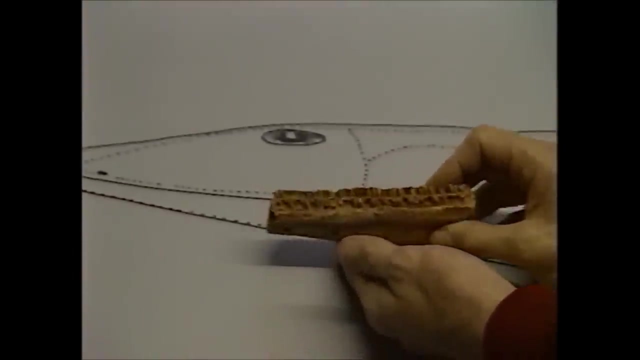 has been studying the earliest tetrapods Music plays. He's trying to find out how and why limbs evolved from fins Music plays. Only 10 fossil pieces have been discovered to date, but even from these few, Eusthenopteron is one of the few fossil pieces. 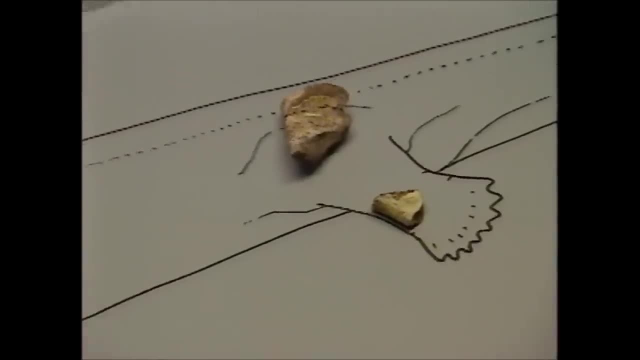 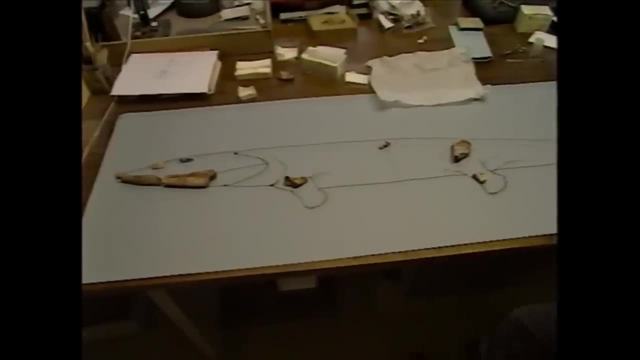 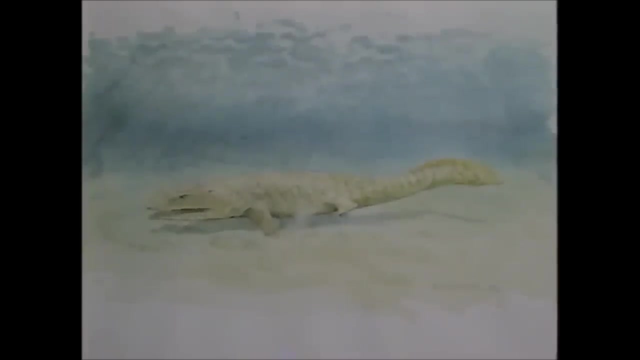 that has been discovered to date Music plays. But even from these few specimens, an image of this new creature is emerging. Music plays Almost five feet long. it looks like today's giant salamander Music plays. I suspect that the reason why limbs evolved. 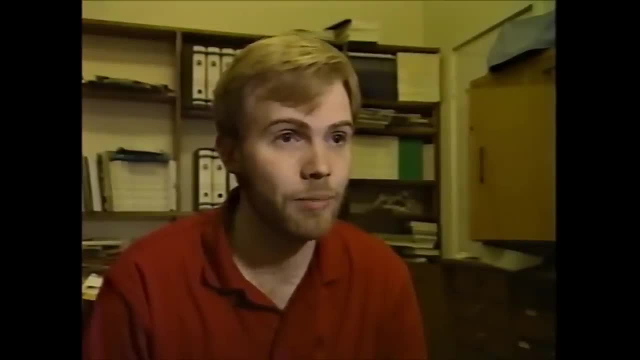 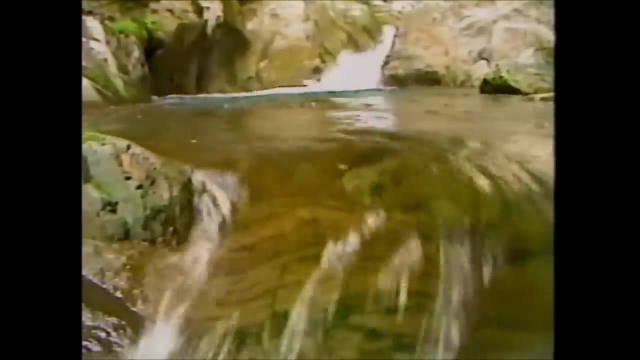 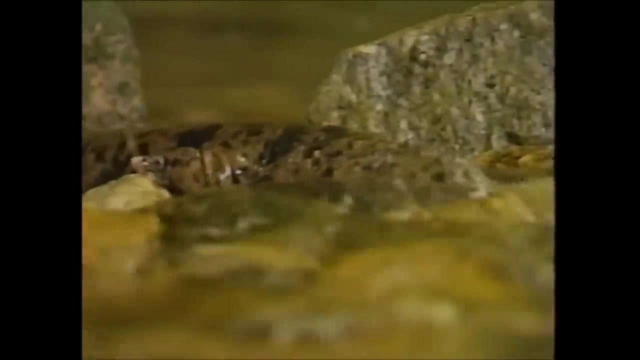 was because these animals were living in very shallow water and limbs can be rather better than fins for moving in those sort of conditions, even if you're not really moving onto land. Music plays These earliest tetrapods, with limbs rather than paired fins, still have gills, tail fins. 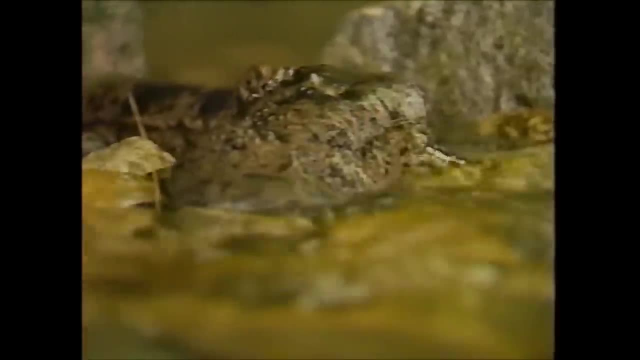 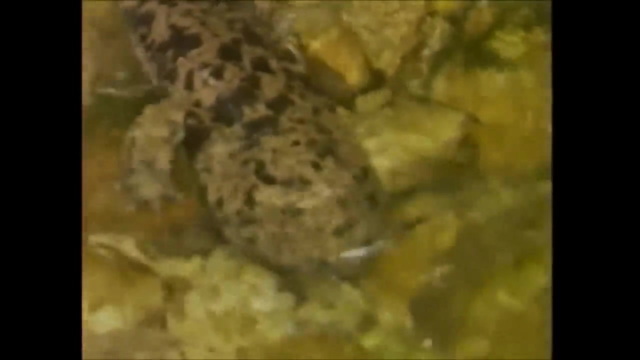 and other features which suggest that they were very much aquatic animals. So I don't really believe that they were using their legs for walking purposefully over land. They might have made short excursions over land, but more probably they were using those limbs in shallow water. 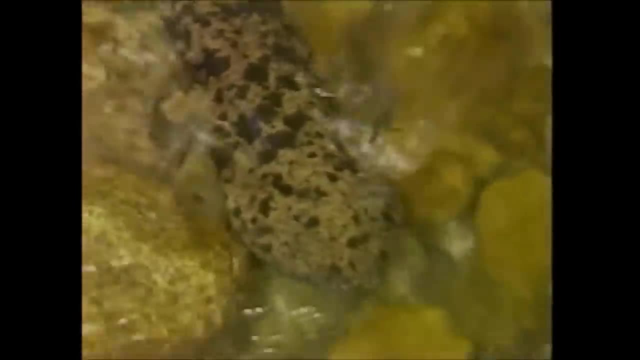 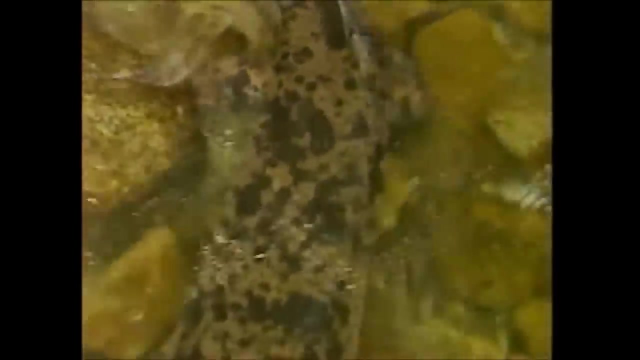 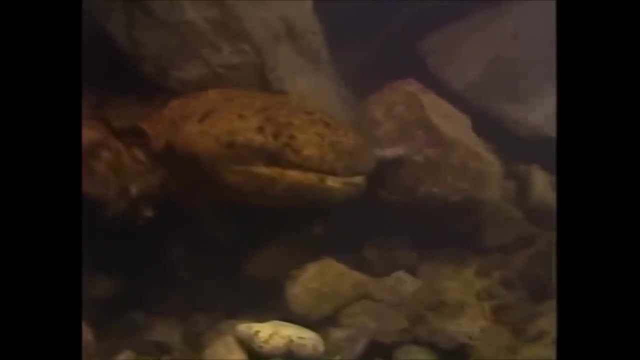 Music plays. Today's giant salamander still spends most of its time in the water. Negotiating the shallows is a matter of walking, not swimming. Music plays Even in swift currents. the salamander plants its feet on the river bottom and moves around with ease. 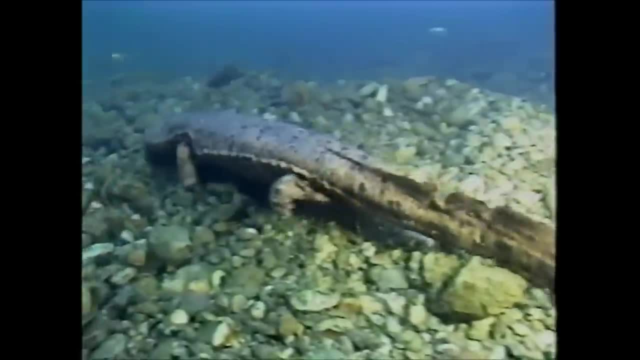 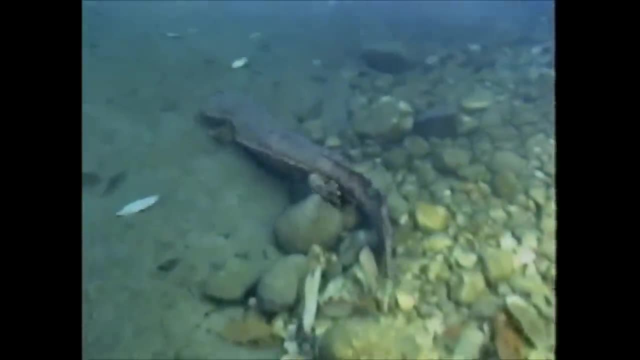 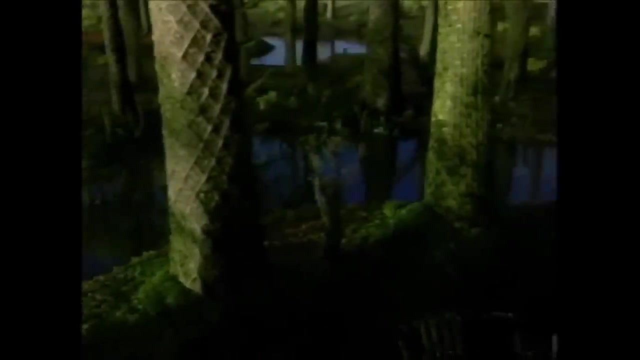 aided by its natural buoyancy. Music plays. To move as fluidly on land the salamander would require a far sturdier skeletal structure. Music plays: The salamander's feet would be as wide as a tree. Music plays 360 million years ago. 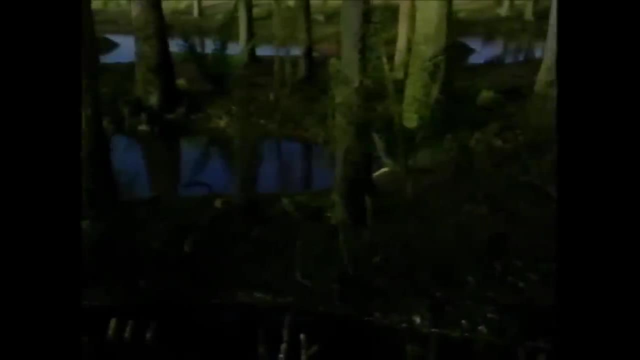 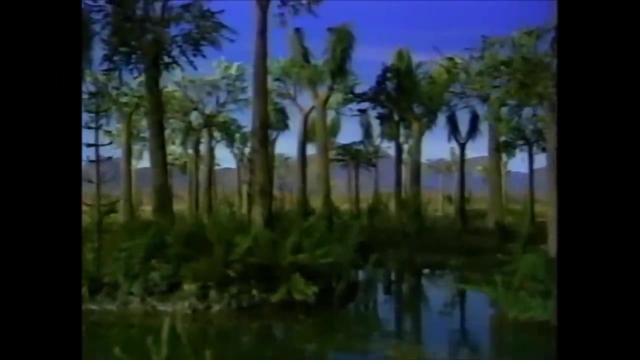 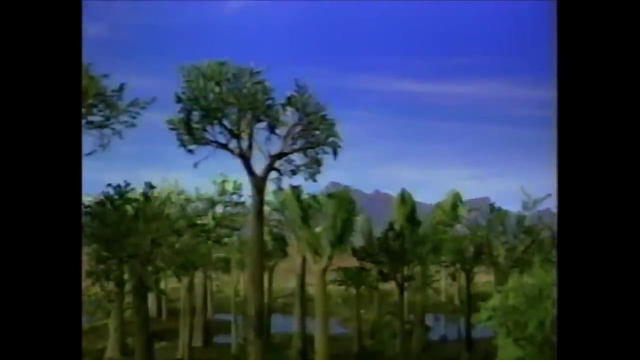 the once barren earth lay under a canopy of green Music plays. Giant forests thrived and small insects now burrowed in the shady wetlands and soil Music plays. This landscape was ready to support new life- Music plays- But to take their first step on land. 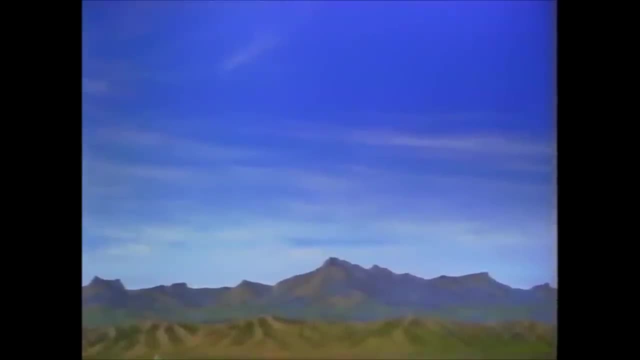 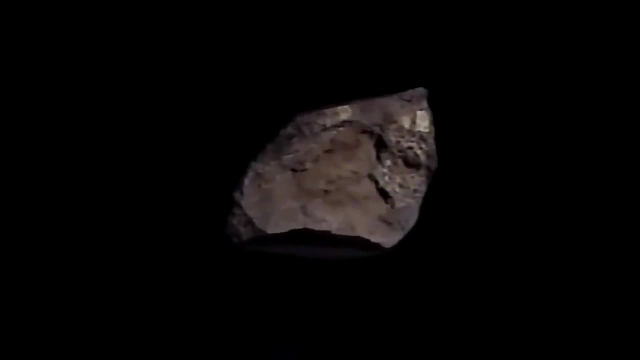 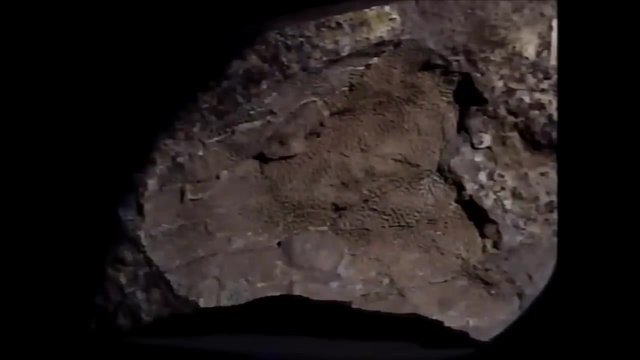 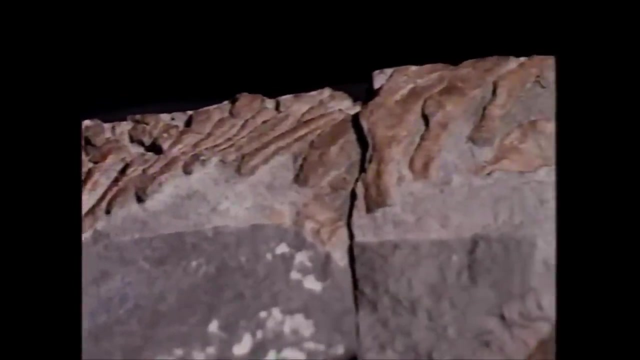 our ancestors had one more obstacle to overcome: gravity. Music plays. This is Ichthyostega, an animal that surfaced 10 million years after the earliest four-legged creatures. Music plays: Judging from the size of its skull, Ichthyostega measured nearly four feet long. 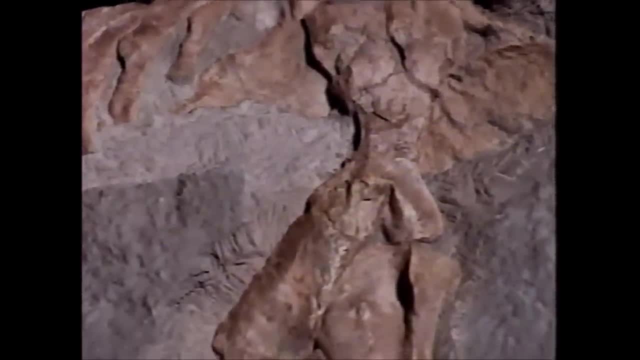 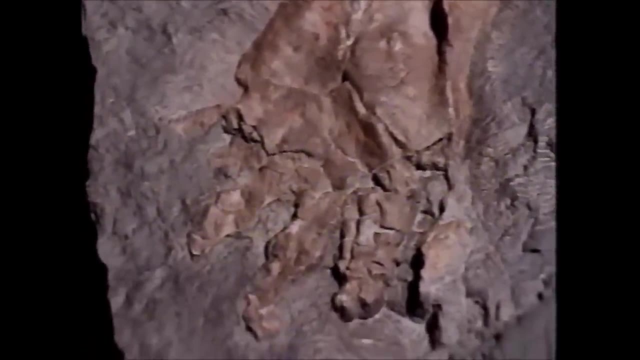 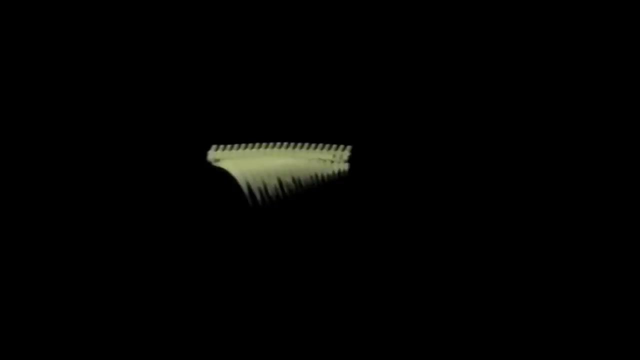 Its backbone and hind legs, clearly defined, Music plays. But this animal also had thick finger bones and a sturdy skeletal structure. Music plays. Scientists conclude this was the first creature to walk on land. Music plays For the first time, an animal with a supporting skeleton around its backbone. 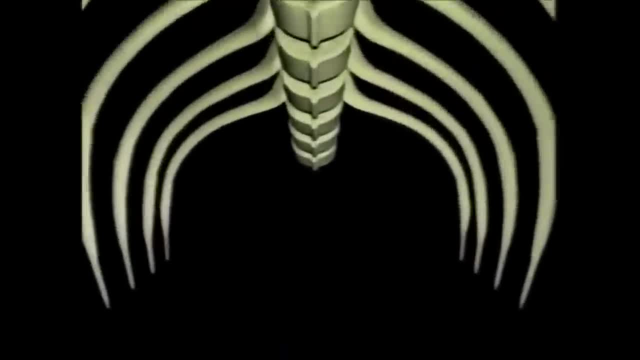 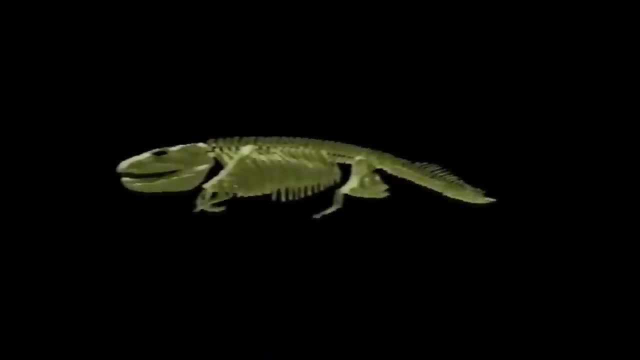 Music plays. The rib cage protected vital organs like the heart and lungs On land. without the buoyancy of water to cushion them, these organs would be crushed by the animal's weight. Music plays By developing ribs, Ichthyostega emerged in a body. 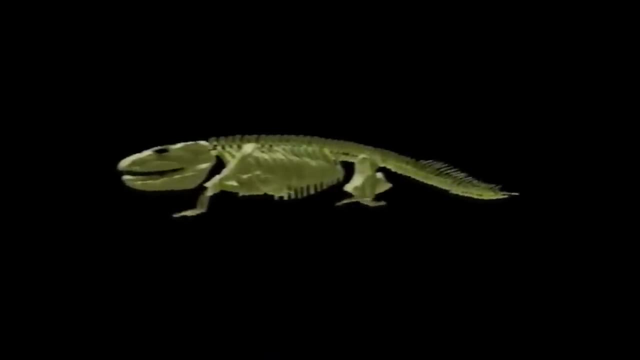 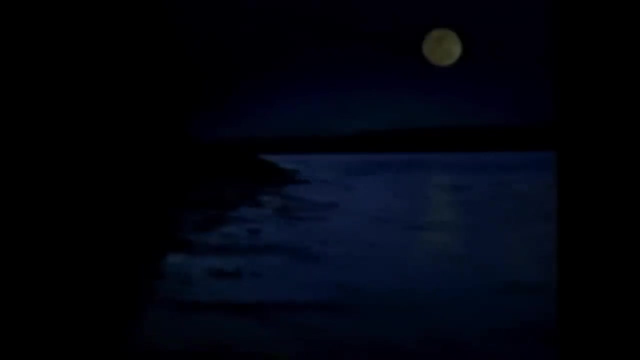 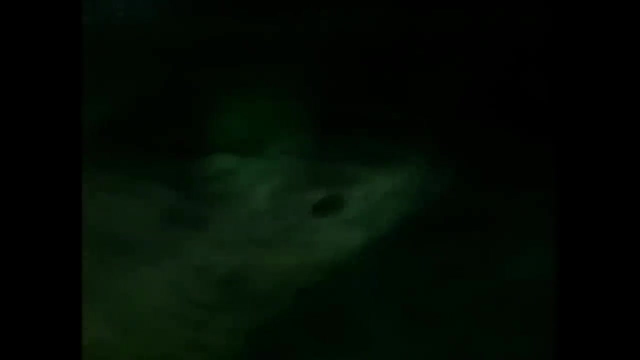 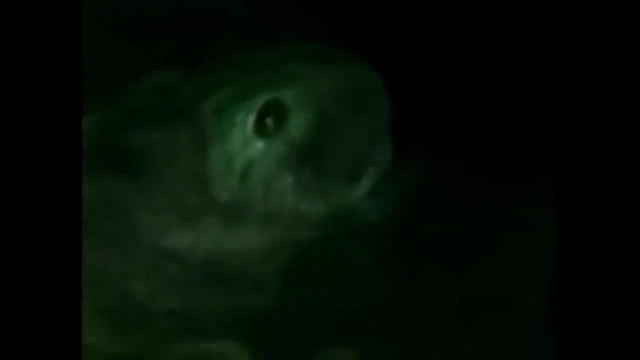 that could withstand Earth's gravity and move about freely over land. Music plays. At long last, the time had come to look beyond the water's edge. Music plays. A hundred million years had passed since the earliest fish ventured from the ocean into freshwater. Music plays.